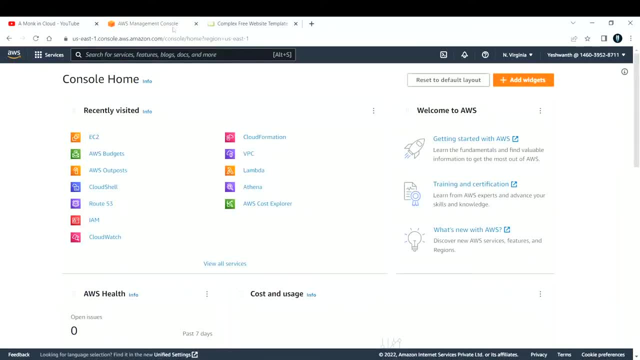 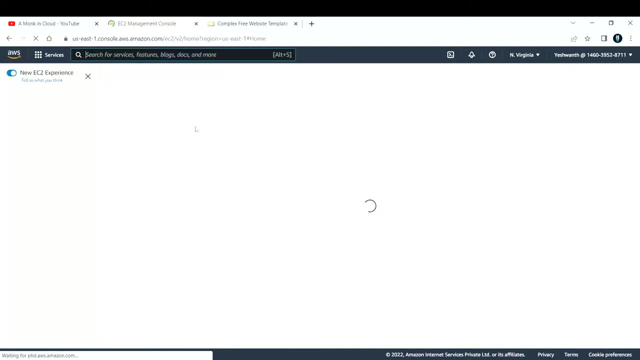 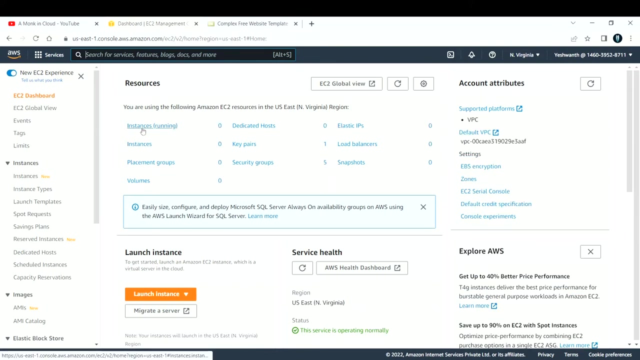 instance. So let me go to Amazon console. So this is my AWS console. So to create an EC2 instance, search for EC2.. So select EC2.. If you see, right now there are zero instances running, Let us create one. Alright, so click on. 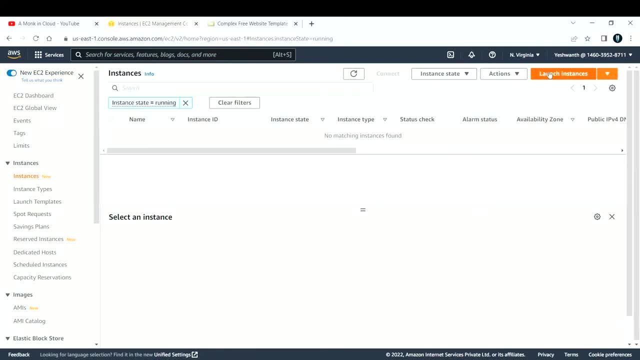 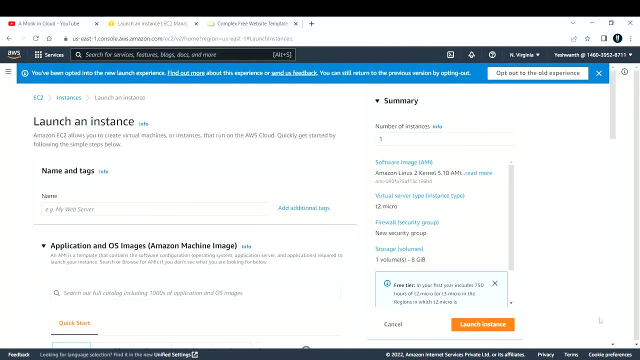 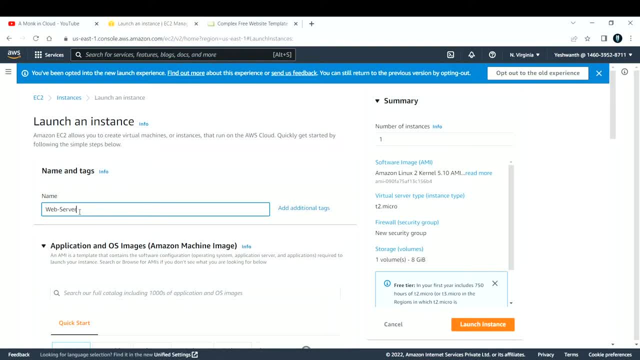 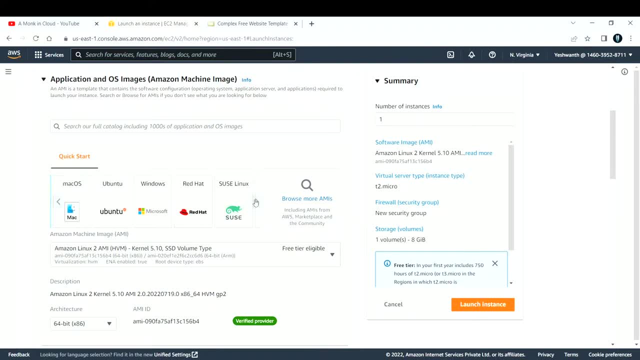 Okay, So I'm naming this as web server. Select the OS that you want. So, for example, there are multiple OS types that you have, but I'm good with Amazon Linux, as this is coming in free tier. Okay, So I'll select Amazon Linux, and this supports 64-bit and 32-bit, So I recommend you to. 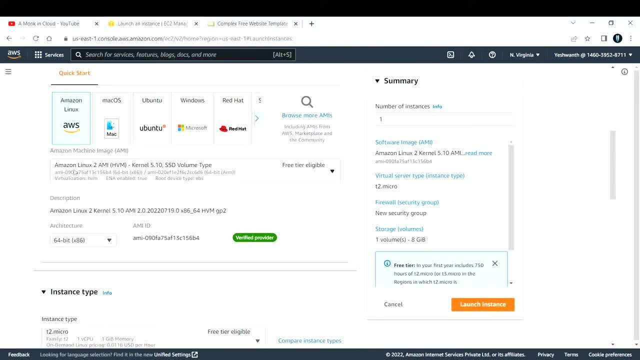 go with 64-bit, Okay, So also make sure that your server is active in your帶. Those are above these wedding sets which you can use to load or let something dark or something like that. So you you are using under free tier if you are not paying as you go. okay, so select the one that. 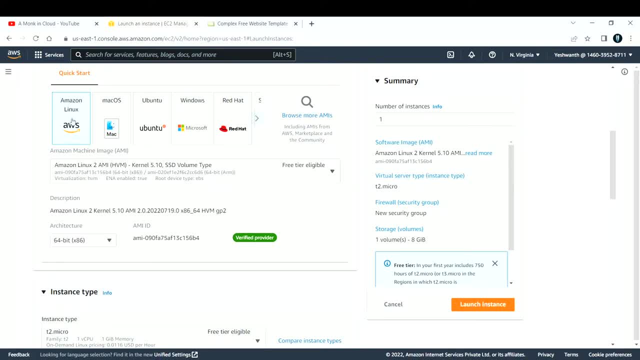 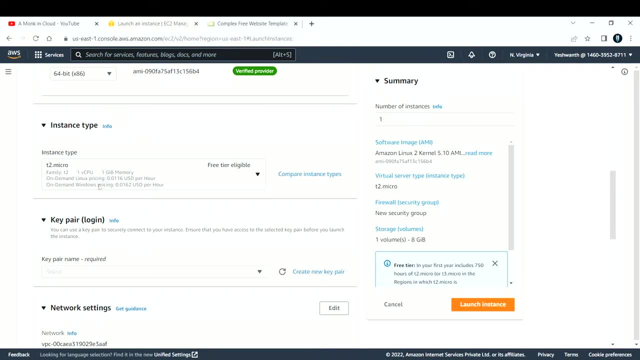 you are using for free. okay, so i'm going with amazon linux 2, and that is available for free, okay. next is again instance type. you need to select the one that is free for you if you are not paying. all right, so i'm going with t2.micro, and even i can go with t1.micro, but i feel that 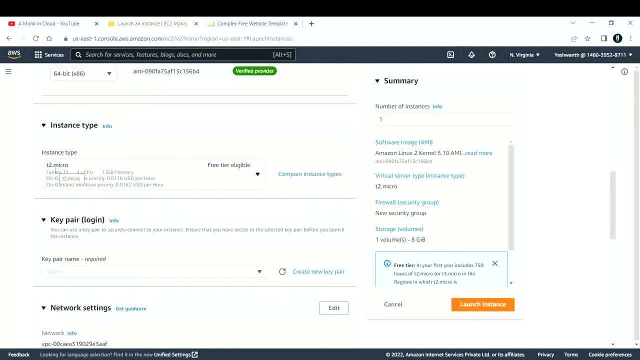 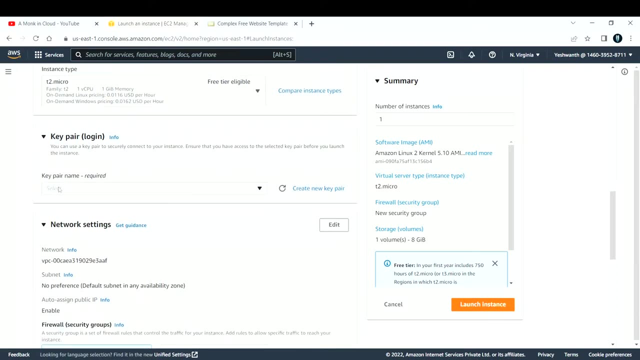 this. that instance type is not, uh, you know, supporting the one that the activity that i'm presenting today. so i'm going with t2.micro and to log into this ec2 instance you need a key pair, all right. so if you have already created it, go with the one, or else you can create new here. 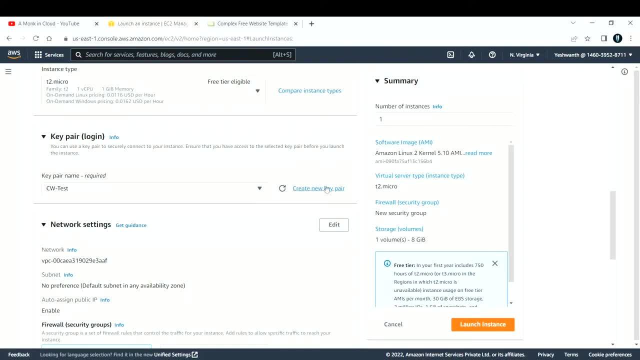 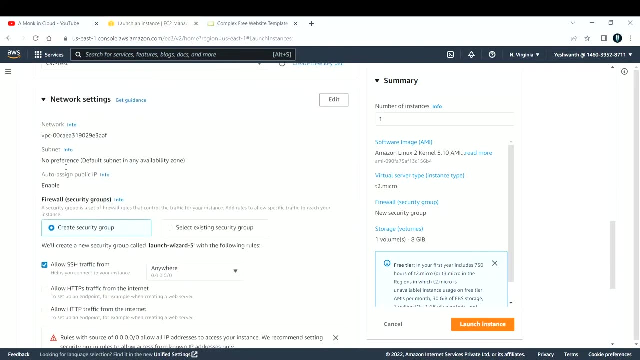 if you do not know how to do these steps, i've explained in detail all these steps about you creating an ec2 instance in a separate video. you can find that in aws playlist. you can go there and watch that video. all right, so i'm good with the network settings. so i'm allowing ssh connection. 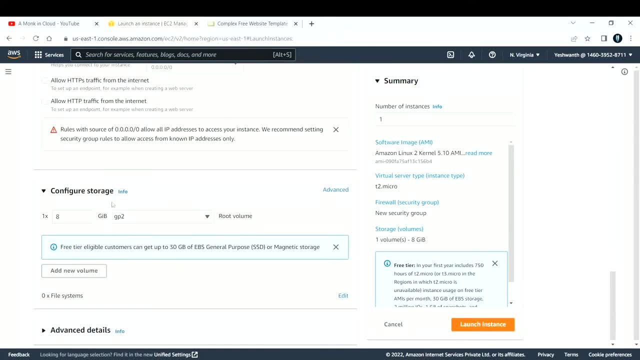 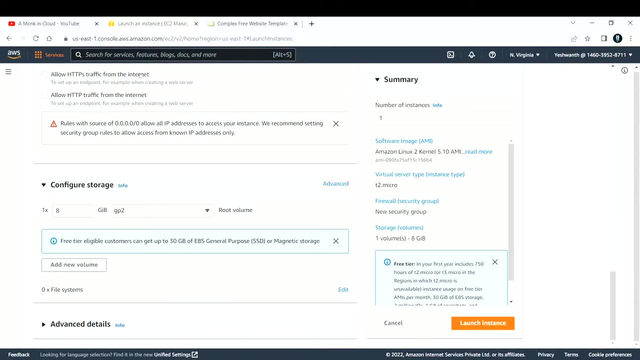 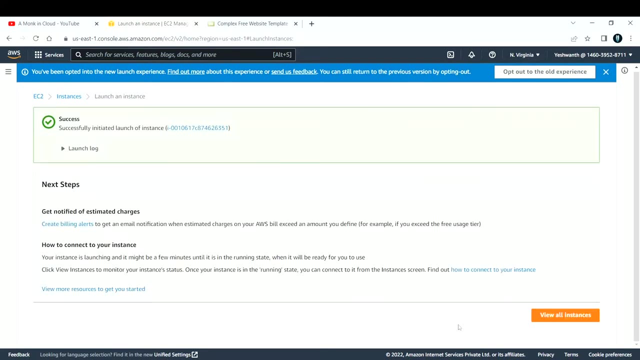 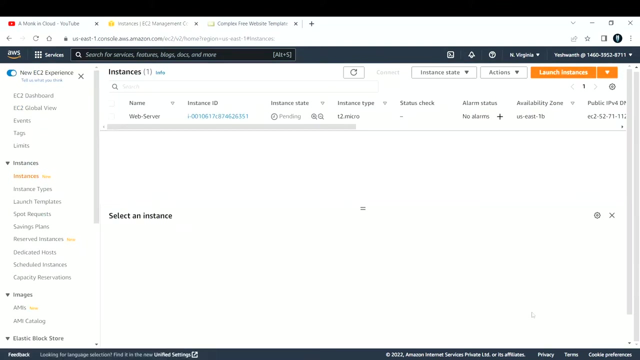 all right, so from everywhere. okay, so i'm good with that. so these are the things that i need to fill in before creating an ec2 instance. i'm good with this. let me click on launch instance so it says success. let's wait for a couple of minutes, so i think it will take two or three. 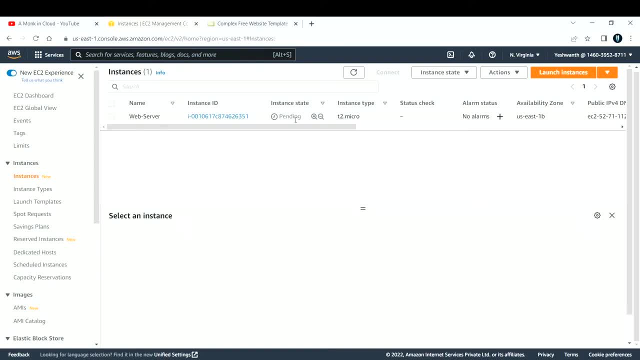 minutes to spin up a virtual machine or ec2 instance, and the instance state should change to running and the status check should be two by two. okay, so we'll meet once the instance is running and the status check is passed. all right now, if you see the same ec2 instance that we created. 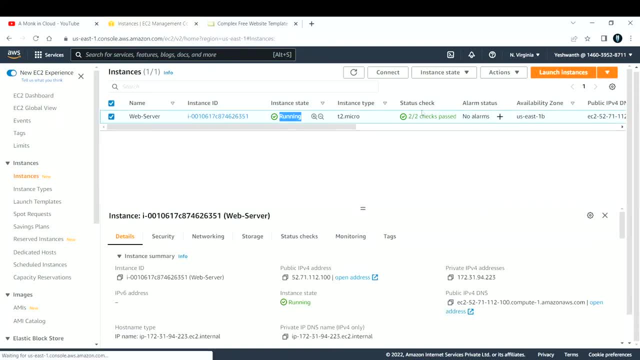 is running, the state of the instance is running and the status check, two by two, passed. okay. so if you see the details of the virtual machine or an ec2 instance, it is like this. okay, so this is the key name that we use and this is the launch time, and these are all the things that we selected. 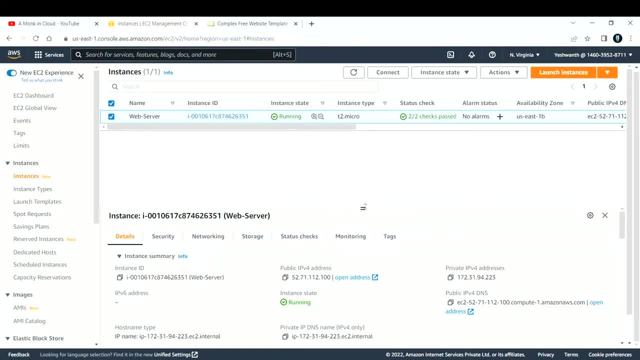 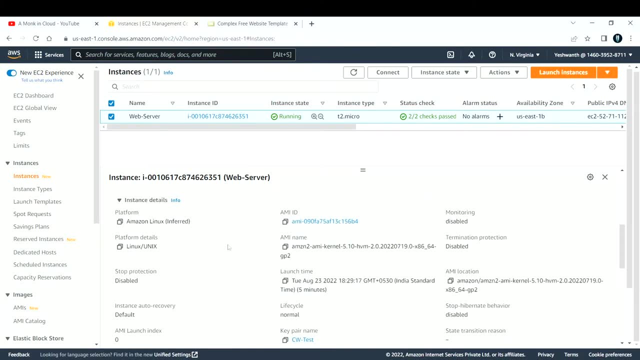 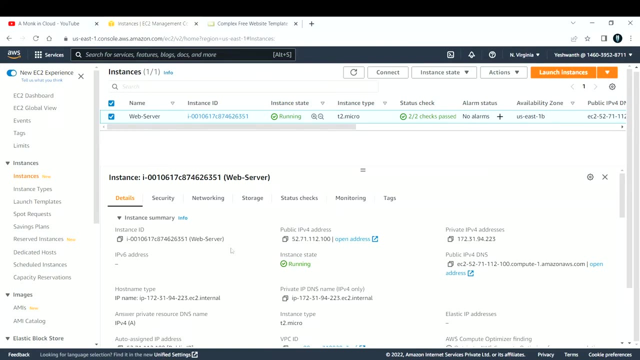 all right. so if you see, if you still want to see the summary of this ec2 instance, you can, you know, open up this. you can check this box and if you see, all the details will be present here. okay, so this is how you create an ec2 instance. the next step would be to connect to this ec2 instance. 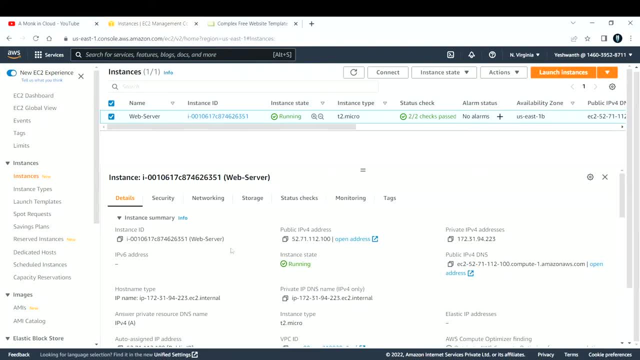 and host your website. so to connect to your ec2 instance, we have many different types and i am going to follow ec2 instance connect method. so if you, if you are not aware, there are multiple ways on how you can connect to this ec2 instance. so if you do not know, please watch my other video. 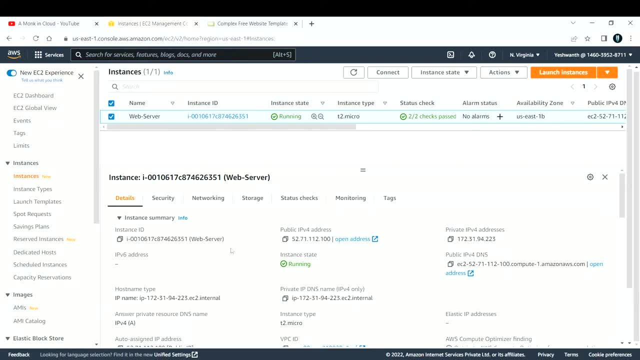 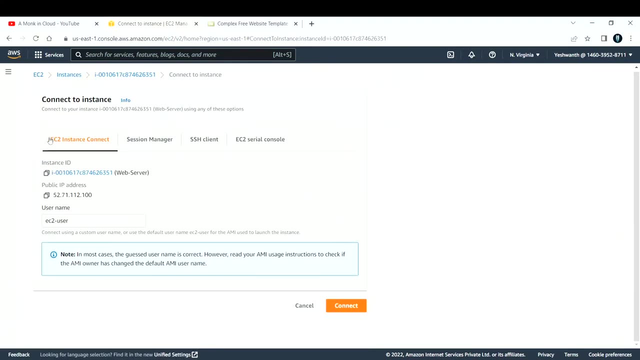 i will drop the link to the other video in the description box below. you can go check that out and then continue here. all right, so i will follow the first method. instance connect method. okay, so to connect, click on connect here. so select ec2 instance connect and click on connect. 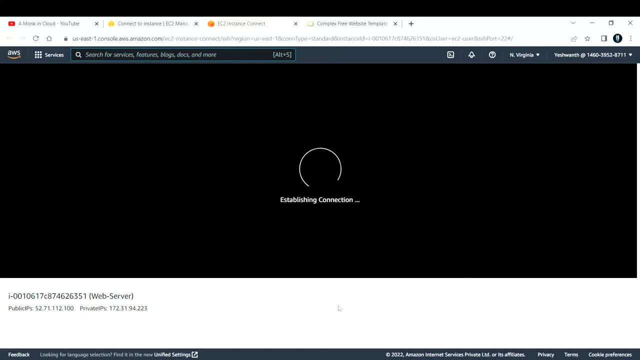 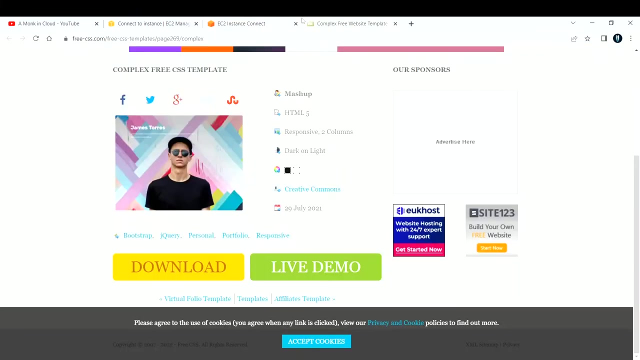 all, right now i'm in my ec2 instance, so i've logged in to my ec2 instance right now. all, right now let us start the hosting of our website. so i have. i i have not written any code right, so what i did is i went to this website and i found a beautiful website, so i'm going to use this. 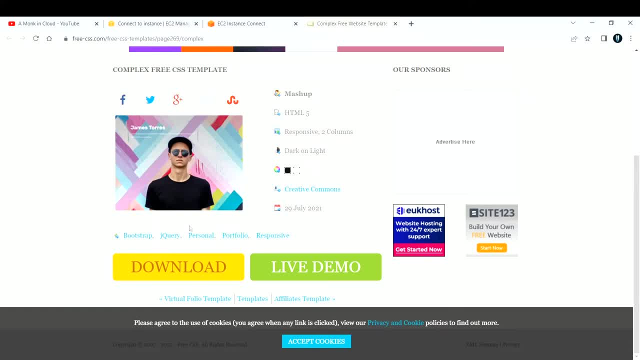 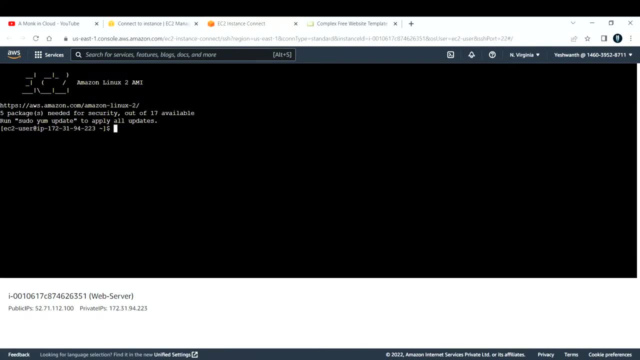 as my personal website and host it on the ec2 instance. okay, so let's see how to do it. okay, so after connecting to ec2 instance, you know, change yourself to a root user. okay, by this is the command sudo, su hyphen enter. so now you are the root user. so first, before installing anything, 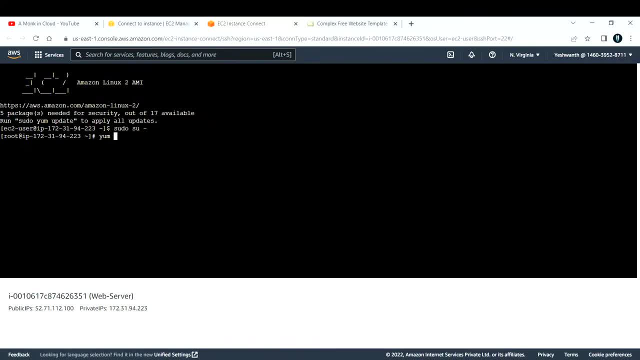 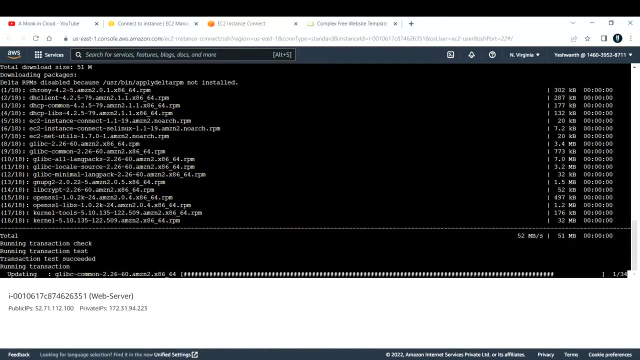 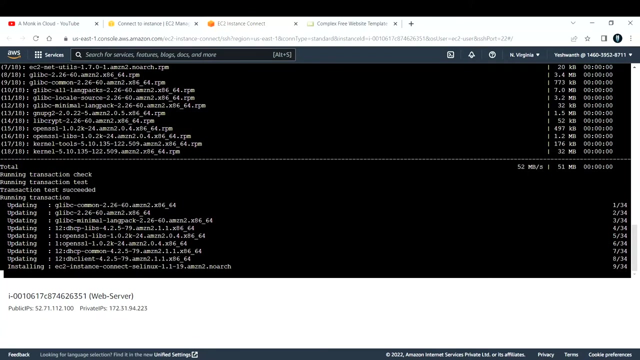 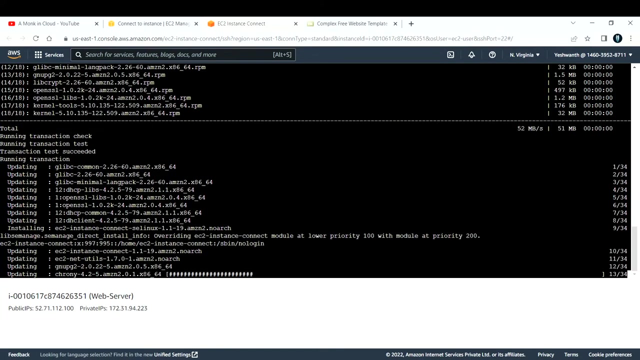 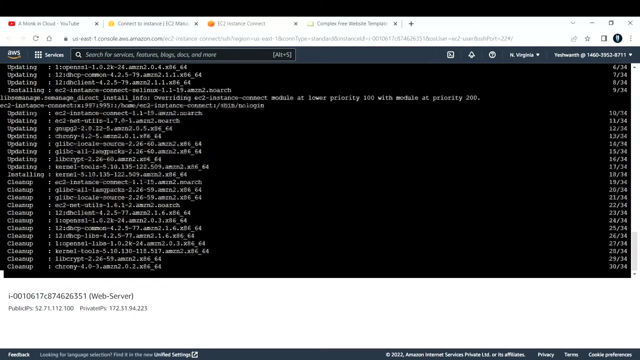 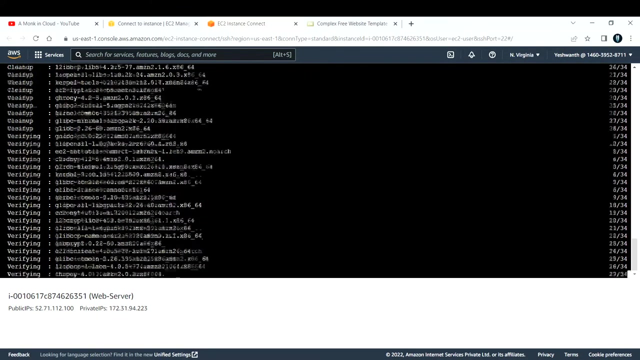 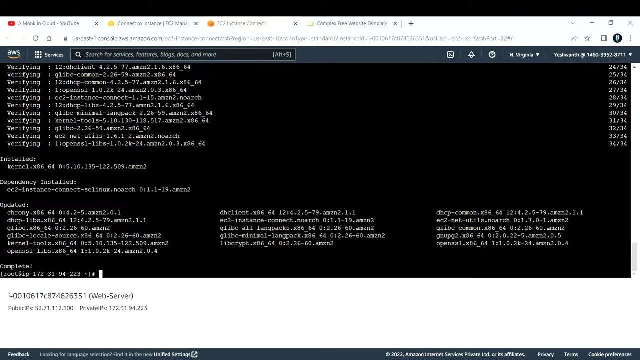 just update the system first. so the command to update is m update hyphen y. okay, so m update hyphen y. so this will take a couple of minutes to get the system updates right now. if you see the system is getting updated, all right, the system got updated. if you see it says complete: okay. so the next thing that we need 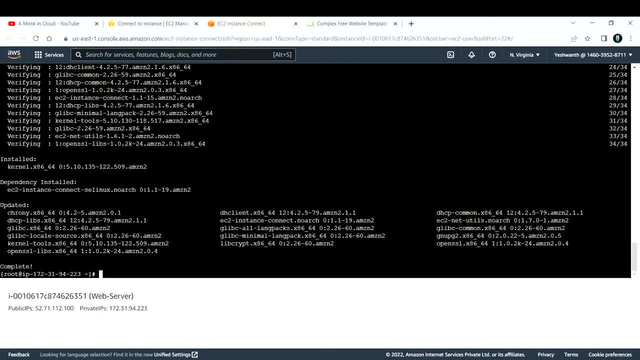 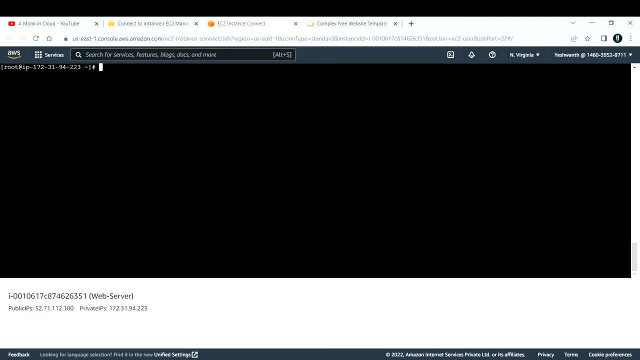 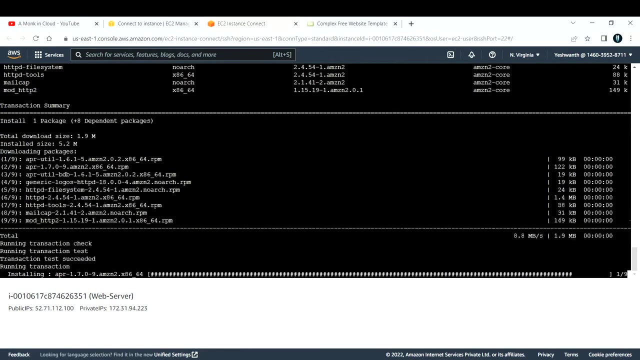 to do is to install httpd. all right, so that is the web server. so to do that, run a command. let me clear the screen. first run this command: yum, install hyphen y, httpd, httpd. okay, hit enter so it will download all the packages and it will install. 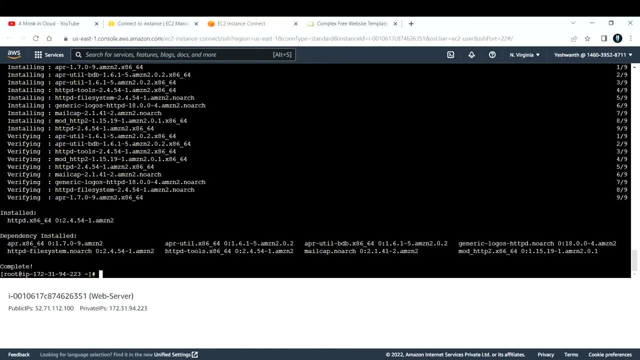 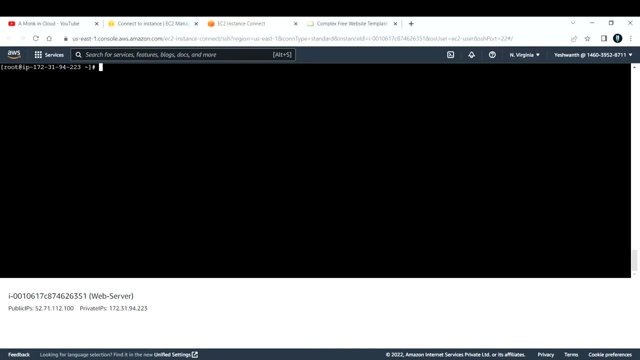 the web server. okay, so if you see complete, all right. so let me clear the screen again. okay, so now what i'll do. i'll check the status of this httpd. okay, to do that. so we have a command called systemctl- status httpd. you see it is inactive. so let us enable this one at the end. but till then, 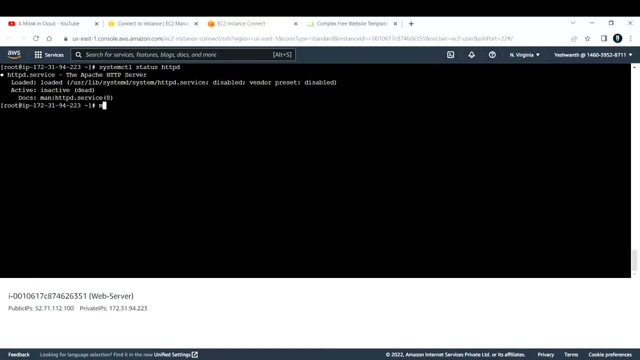 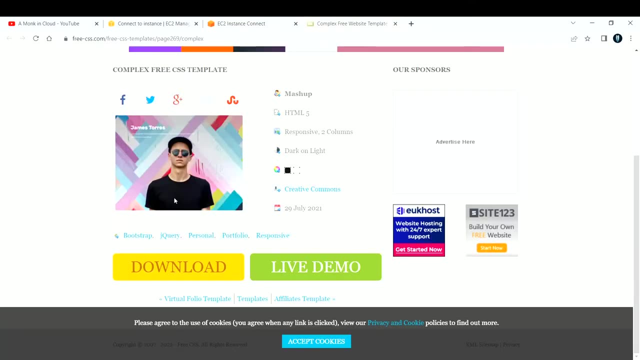 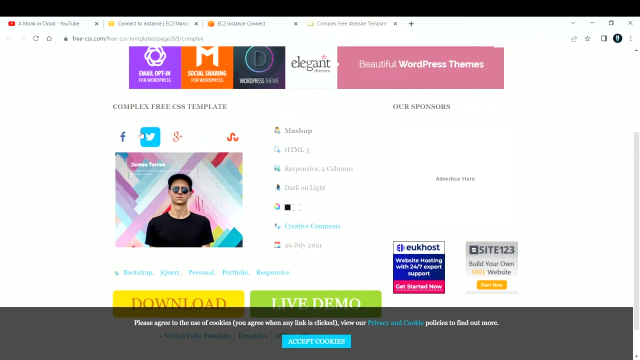 let us, you know, create a directory and name that as temp. let us get into that folder, okay. so now what i'll do. i'll get the zip file of this one, this website. so this is the website that i'm going to. you know use. this is available in this one, freecsscom, so you can also get any of the sample website from. 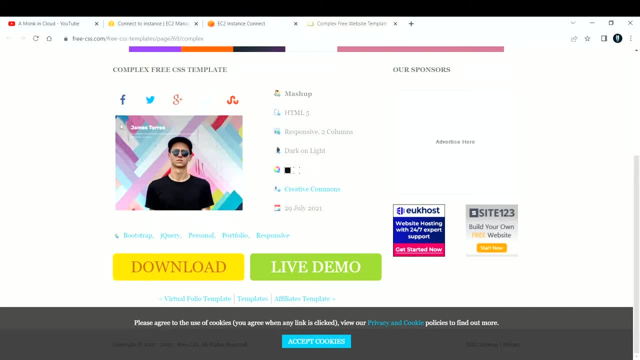 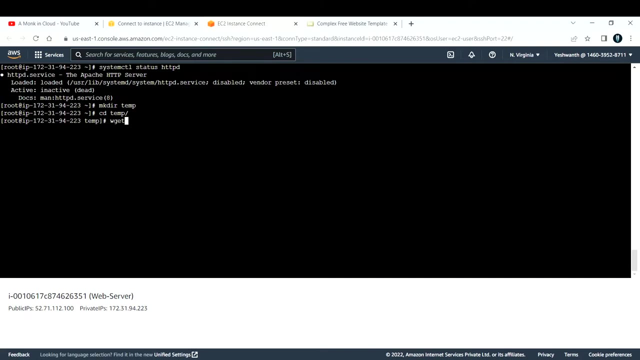 here and host it on ec2ncom. so now i'm hosting this particular website. to copy the link, so just right click copy link address. okay, go back to your ec2 instance. there is a command to download it. so the command is: wget and paste the link that you copied. okay, so wget and the link that you copied. 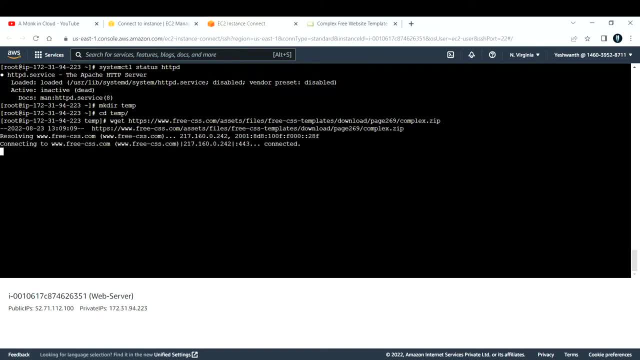 it will. it should be a zip file, okay, so hit enter it, downloaded it, okay. so let's check if it is a available. hyphen ls, hyphen lrt. if you see complexzip is present, okay, let me clear the screen first and rerun lslrt so this complex dot zip file is present first. let us unzip that okay. 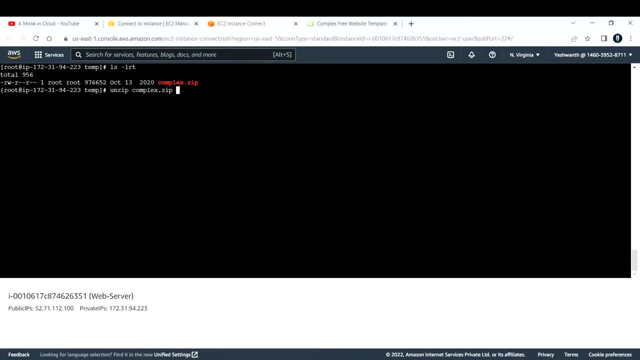 so the command is unzip complexzip. okay, hit enter so it unzipped everything. so let me do ls hyphen lrt and then hit enter and we can see that we have a complexzip and the command is unzip complex, dot, zip and then hit enter so it unzipped everything. so let me do ls hyphen lrt and i will go to my不用. and here it is the command from this one, and i will be writing a command for how i want this file, so i'll just hit create, ending, and here you'll see it. so it's like a very simple command. so let me do use the command from here and i'll put in my use to avoid any other words, if you have any. 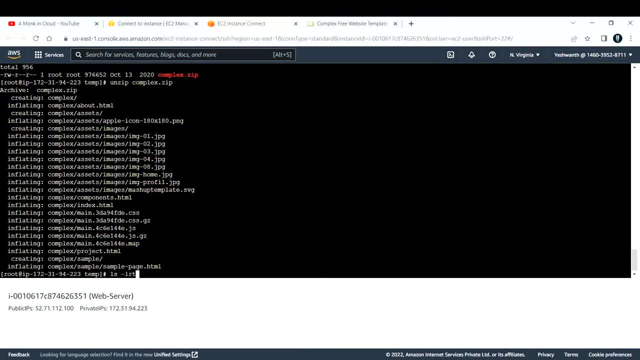 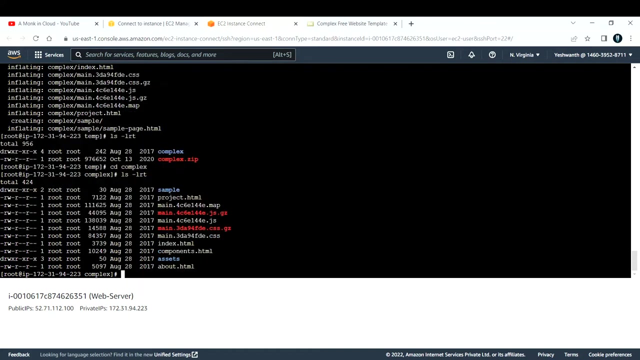 so let me do ls hyphen lrt again. now, if you see there is a folder called complex and there is another zip file called complex, zip- okay, so let's see what is there inside. complex- okay, so i'll get into that cd. complex- okay. so now ls hyphen lrt. you see these are the html files and styling. 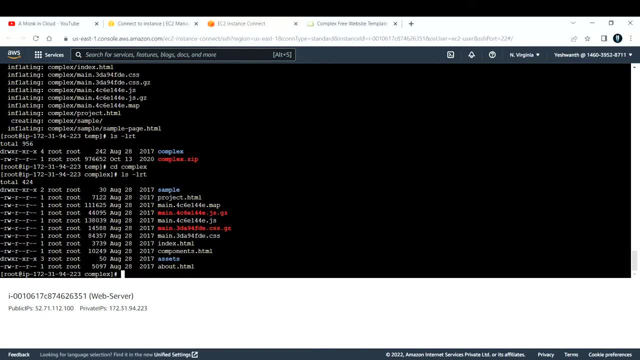 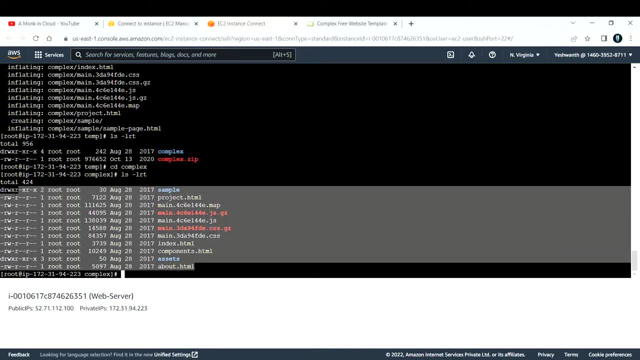 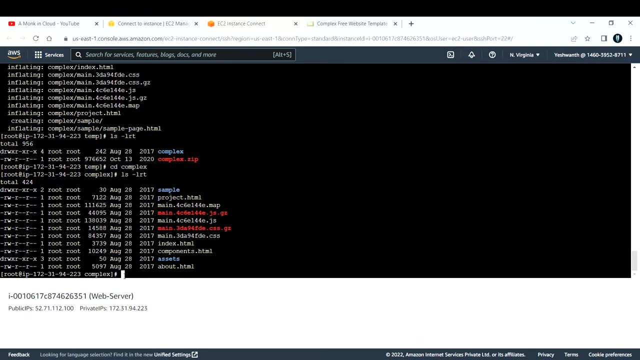 javascript. everything is there inside that folder. so to convert this, you know, into this server, into a web server, you need to move these things, these file, html files and everything into a sub right directory called slash, war, slash, www, slash, html. okay, so let us move all the file from here. 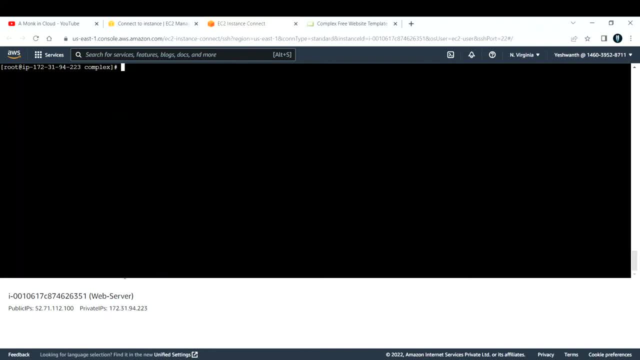 to that particular directory. okay, first let me clear the screen. the command is mv star, move star. star means move cop, move this entire files that are present in this directory to destination directory is war www. slash again html and slash enter. now let us go into slash var. slash www slash html. 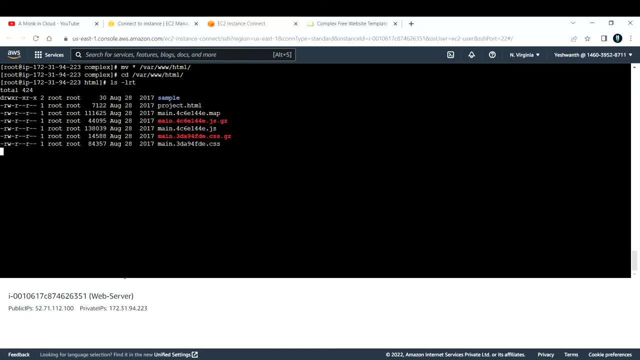 ls hyphen lrt. now, if you see, all these files are transferred to var www html. okay, so this is how you can use this for hosting a server. like you know, host a server on ec2 instance. to check if everything is working fine, let us do one thing. let us copy the public ip address from here. 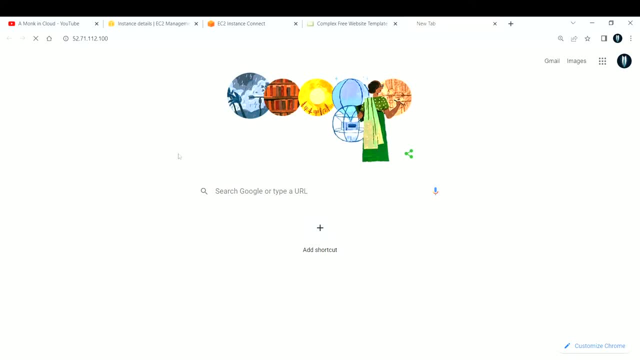 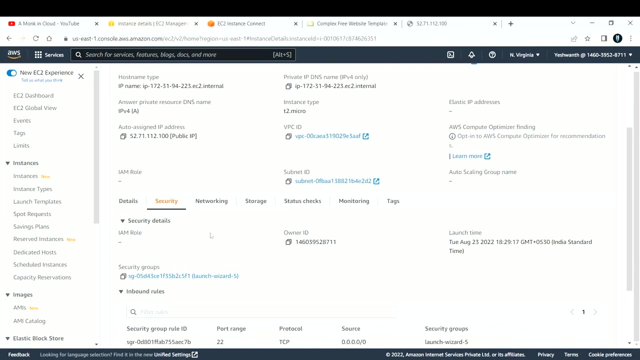 and paste it in the browser. so if you can able to see the content, then everything is working fine. so if you see it is refreshing, refreshing and it is keep loading, that means there is some issue with. so the firewall in AWS is security group. so let us check the security group, let 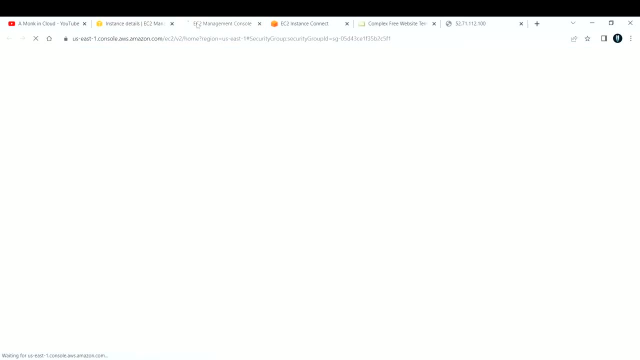 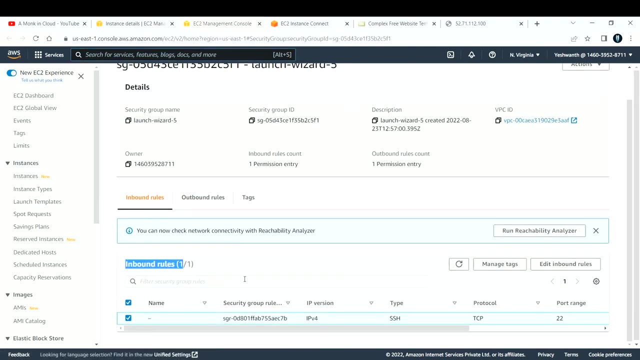 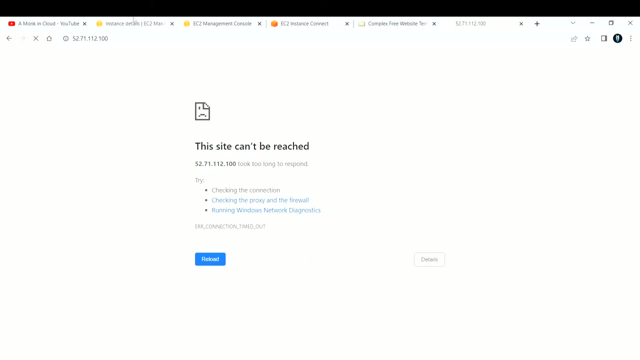 me go to security and open the security group. if you see, in the inbound rules I am just allowing SSH type of connection, but this is a web server, so if you see the site can't be reached, that means we are. we have not allowed HTTP and HTTPS. 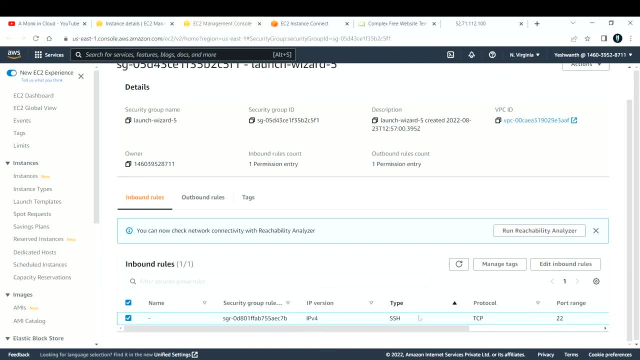 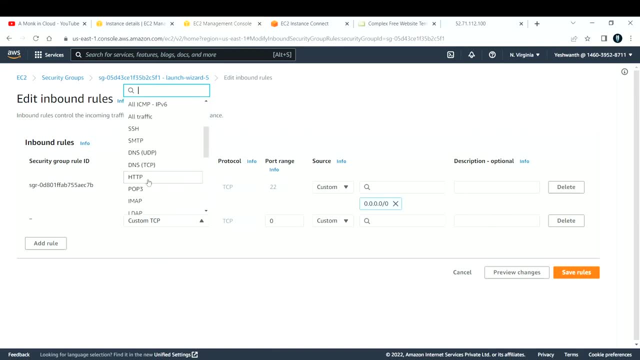 in the inbound rules or the firewall. so let us add those rules here. edit inbound rules. click on add rule. add HTTP. so the port number is 80, as you all know, and I will allow from everywhere. yeah, I'll just say web port. okay, let me add another rule again for HTTPS. so you need to go you. 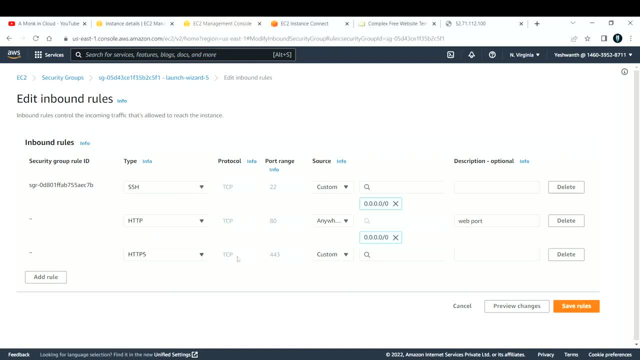 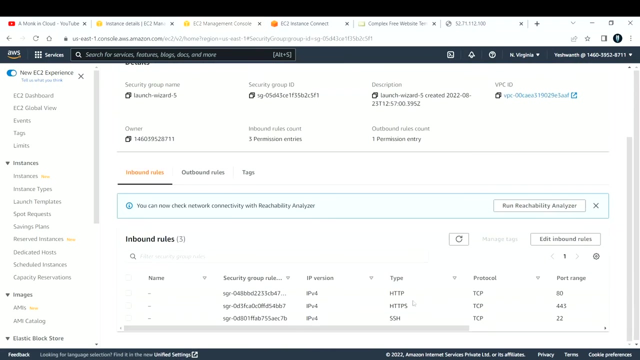 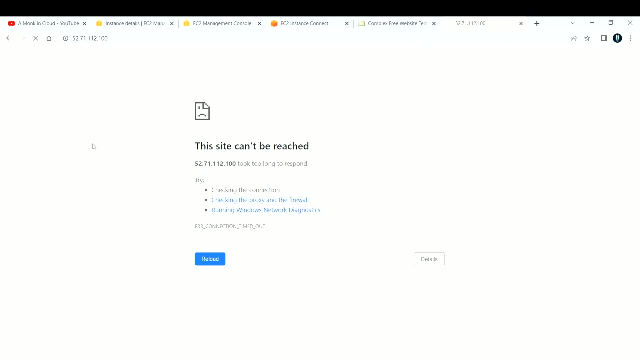 need to allow both of them. if HTTPS and HTTPS, you are not present here, you can add your custom port also. so HTTPS port is 443. okay, I will allow from everywhere again and I will say the same description: web port and save the rules, you, ok? so now we have added HTTP, HTTPS and SSH. now let us go and refresh, if you see. 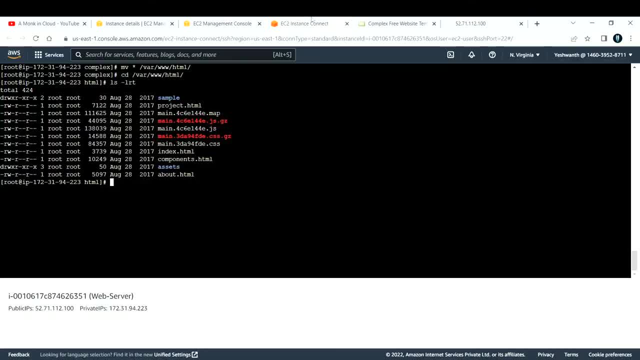 we are still facing the same issue. so the issue is: we have downloaded the web server, but we did not start the service right. so we installed HTTP D, but we did not enable or start the HTTP D. so if we remember, let us check the server and we. 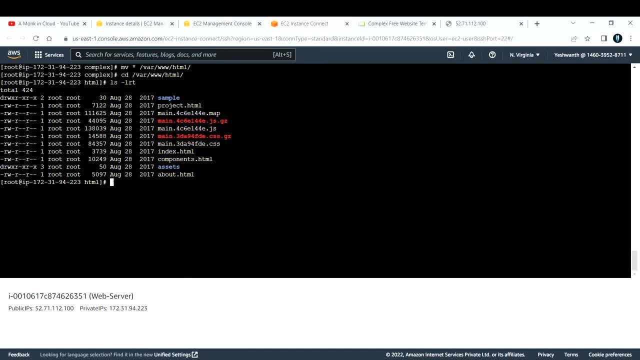 know we can add HTTPS, so we can do such things as well. now let us check the status again. if, if by using the command systemctl, systemctl status HTTP D. so if you see it is inactive, right, so let us enable it first. so the command to enable is systemctl. again, enable httpd. 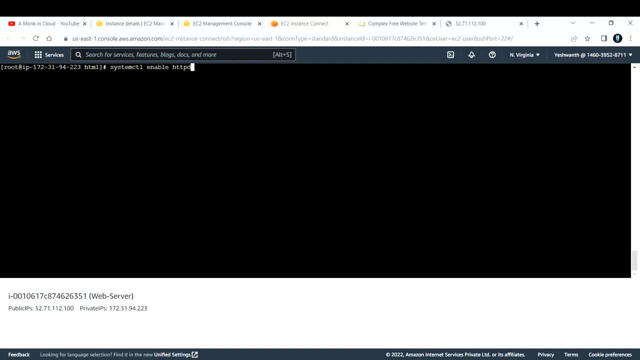 now, if you see it, creates just a 15 of our Azure service themselves. and this of now, if you see it, created a sim link. okay, so now let us start the service. so the command to start is also similar: instead of enable change it to start, hit enter now. if you check the status,